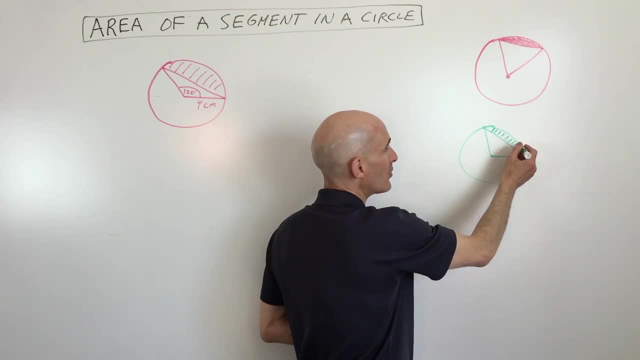 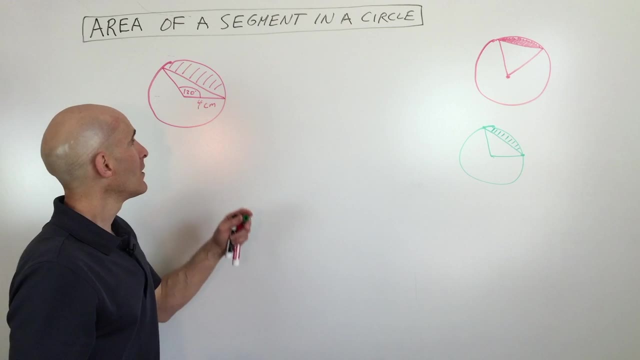 line segment: the area in between the triangle and the outer edge of the circle that's called a segment. so let's do an example so you can see how to do these problems. I'll show you two different ways to approach it. okay, so this one. we're trying to find the area of this segment right here, the dashed. 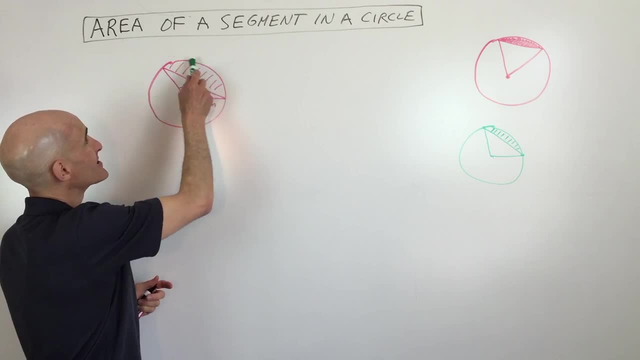 area. so first thing we want to do is we want to find the area of the segment, and then we want to find the area of the segment, and then we want to find the area of the sector which is that pizza slice, that section of the circle. so what we're going to do is we're going to look at the equation of a. 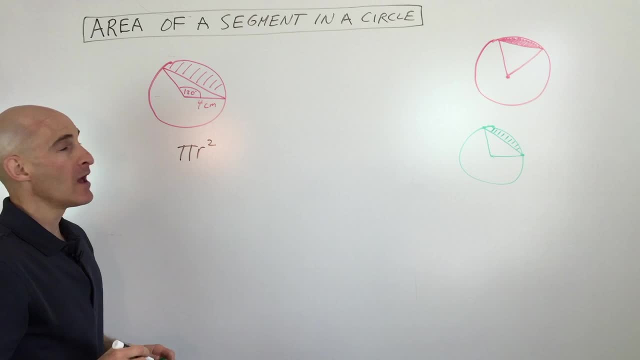 circle PI R squared. okay, what we're going to do is we're going to multiply by 120 degrees divided by 360. okay now, why 120 degrees divided by 360? well, this is actually this region, right here. let me see if I can draw it right here for. 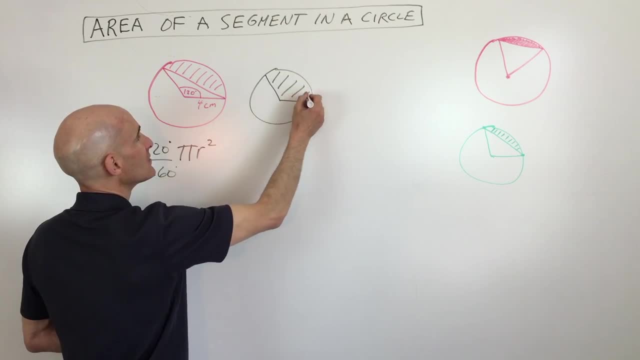 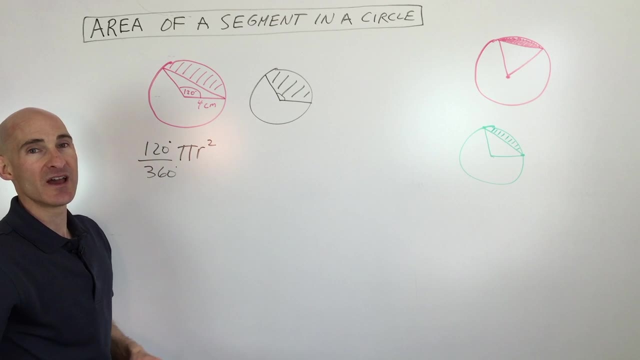 us. this region right here is actually one-third of the entire area of the circle. so I'm just taking the ratio of this central angle, 120 degrees, divided by the whole circle- 360 degrees, to get the area of just this section, that sector. okay, so if we continue that on, we 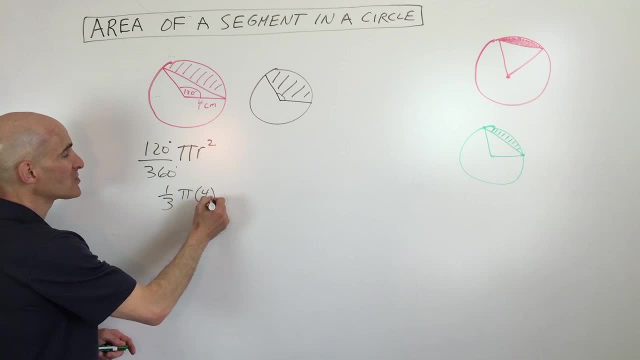 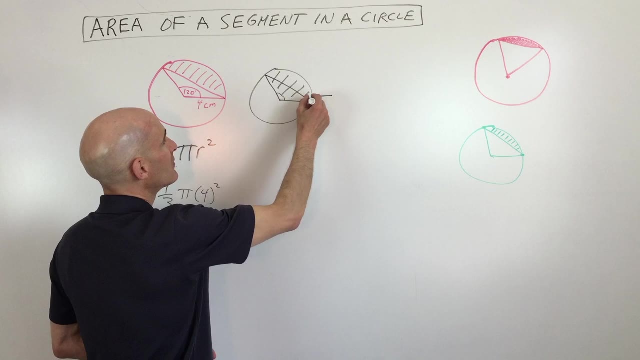 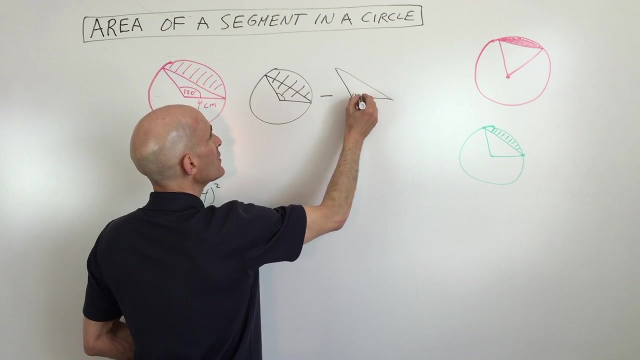 have here one-third times pi 4 squared. okay, so that's this area here. now, what we want to do is we want to subtract off this triangle right here. okay, so if we look at that triangle, let's look at what we have. we have a hundred and twenty degrees. this is 4, and 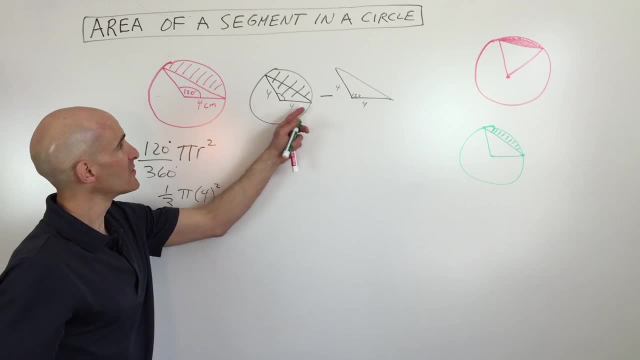 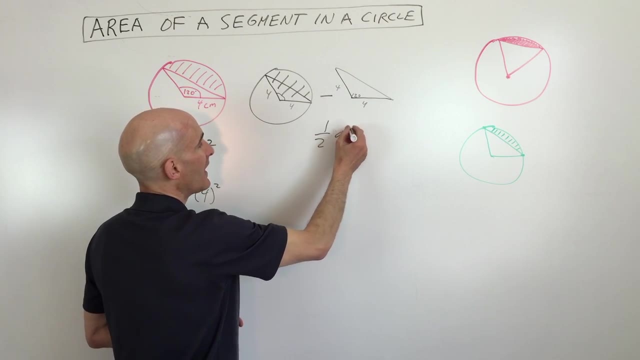 this is four because these are both the radii of the circle, in case you're with me so far, and we want to subtract off this area. now there's a formula you can use and it's one-half a, B sine C, so a and b are the side lengths that make up. 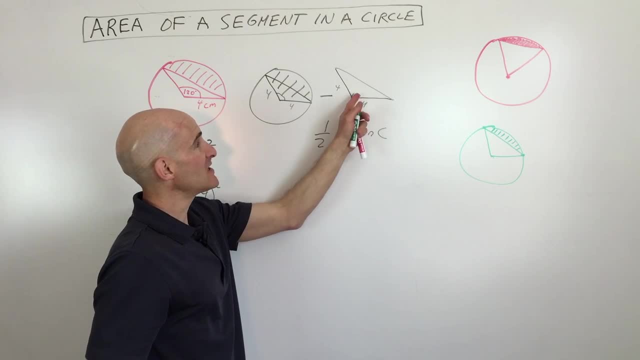 the sides of this triangle and angle C, as the angle is in between the two radii there, okay, in between the two sides. can we think? well, two times 20 degrees, and could that? so we can use this formula, or what we can do is we can subdivide this triangle, okay, into two. 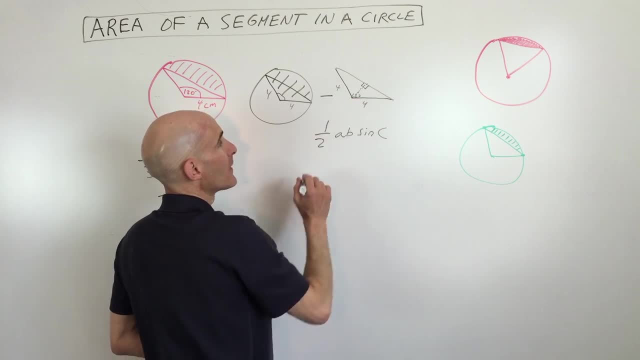 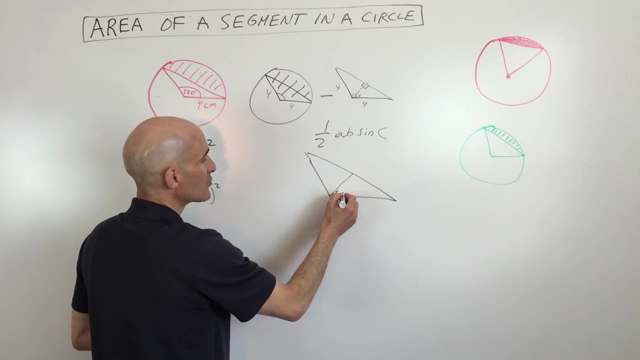 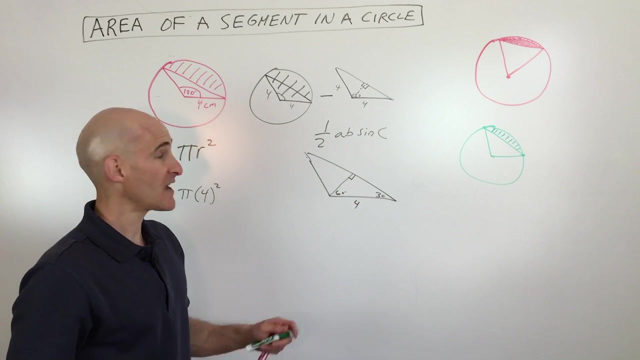 triangles. so what I'm doing is I'm dropping a perpendicular, like so okay, now what I have is: I have- let me see if I can blow this up here a little bit larger for us is a 60 degree angle, okay, like so: this is 4, this is 30, this is 90. so we have a 30, 60, 90 special right triangle. so if 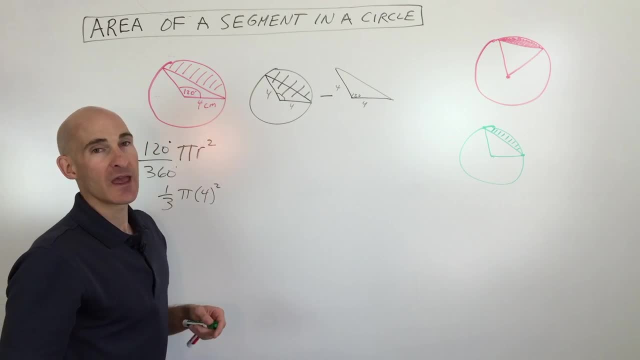 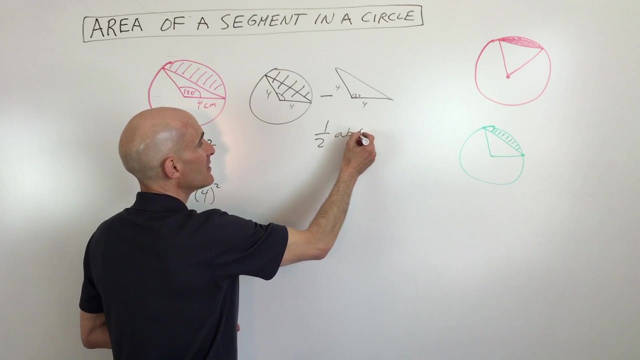 these are both the radii of the circle, in case you're with me so far, and we want to subtract off this area. now there's a formula you can use and it's one-half a, B sine C. so a and B are the side lengths that make up the sides of 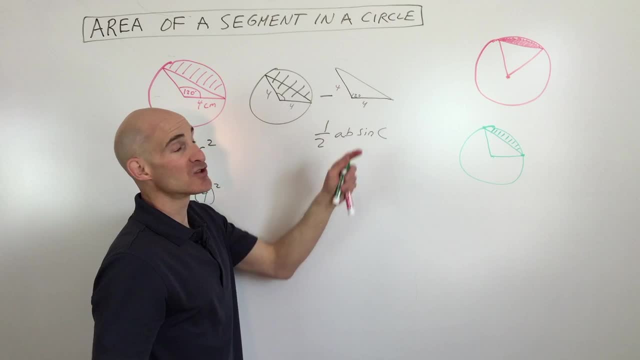 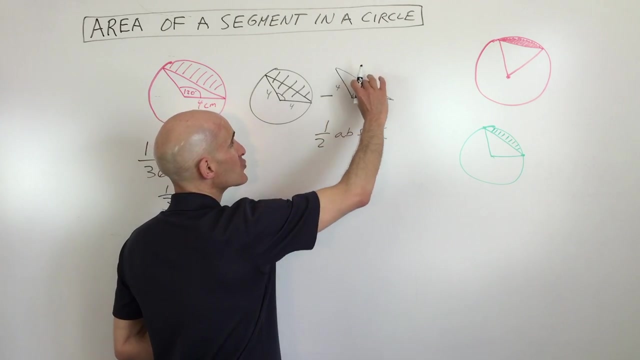 this triangle and angle C is the angle that's in between the two radii there, okay, so in between the two sides. so we can use this formula, or what we can do is we can subdivide this triangle, okay, into two triangles. so what I'm doing is I'm dropping a perpendicular. 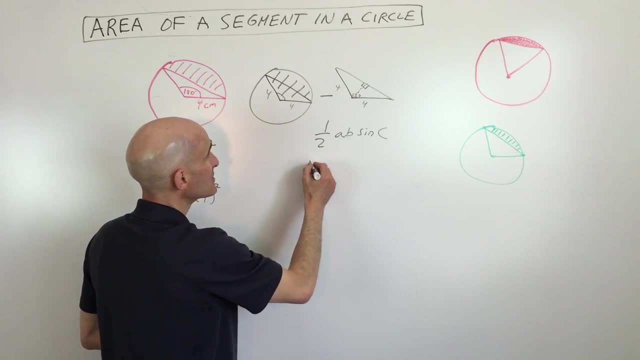 like so, okay, now what I have is- I have- let me see if I can blow this up here a little bit- larger for us is a 60 degree angle. okay, like so: this is 4, this is 30, this is 90. so we have a 30, 60, 90 special right triangle. so if the hypotenuse is, 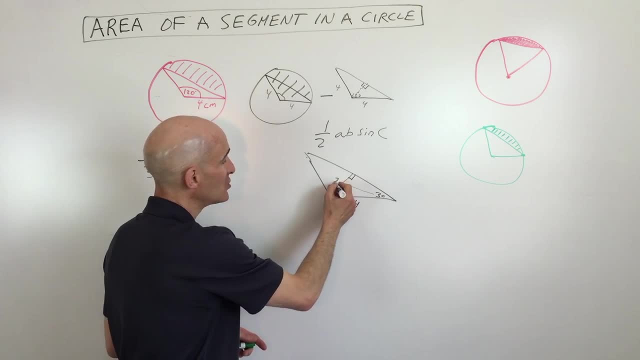 4: the side across the angle which is drawn across from the 30 degree angle. that's going to be 2, ok, and then the one across from the 60 degree angle. that's going to be 2 square root of 3. ok, this triangle is the exact same, so this will also be 2 square root of 3. so 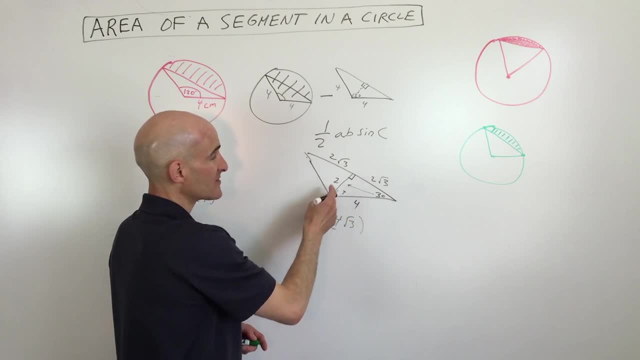 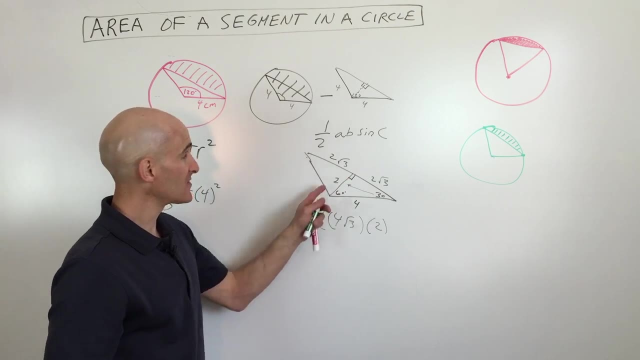 what we have is we have the base, which is 4 square roots of 3 times the height, which is 2 times 1 half. ok, so that's the base times the height, times 1 half, because that's the area of this triangle. so that's going to be. 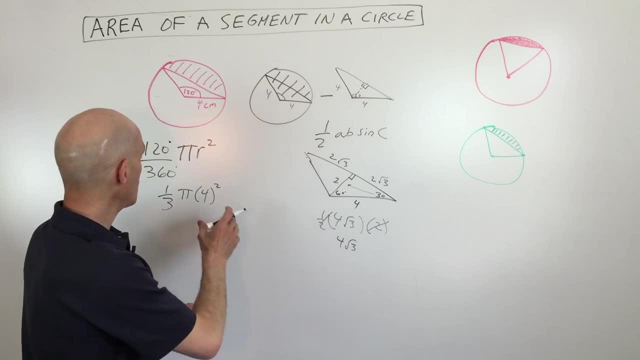 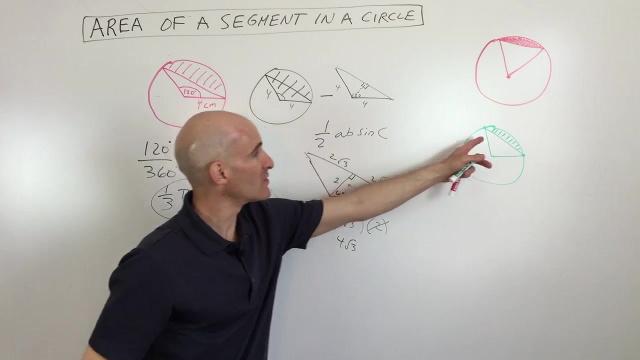 4 square root of 3, cancel. so all we have to do now is take this, the area of the sector, okay, this whole pie slice, minus the area of the triangle, which is four square root of three, and that's going to give you an exact answer. that's going to give us the area of the segment, just this little piece, right. 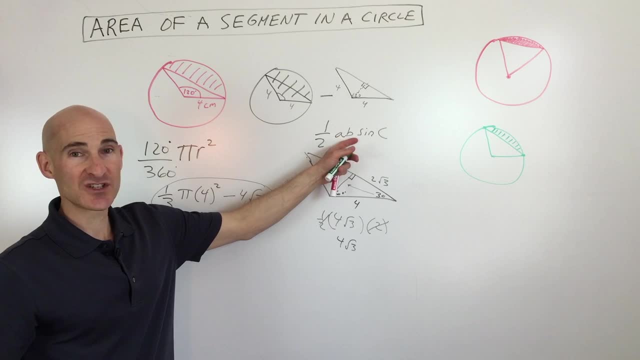 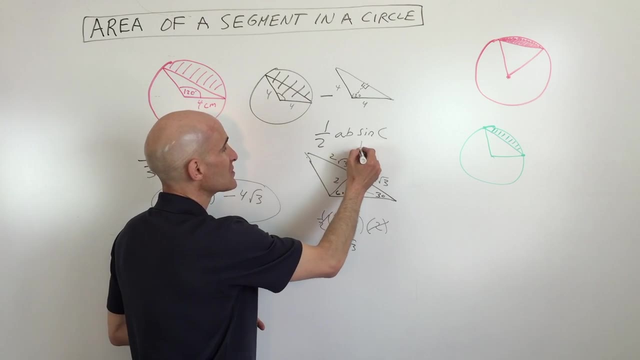 here. so you can either use this formula, like i was mentioning before, or you can use the method of just splitting the triangle in half by dropping a perpendicular. let's look at this real quick. this is one half four times four times the sine of 120. sine of 120 is square root. three over two.